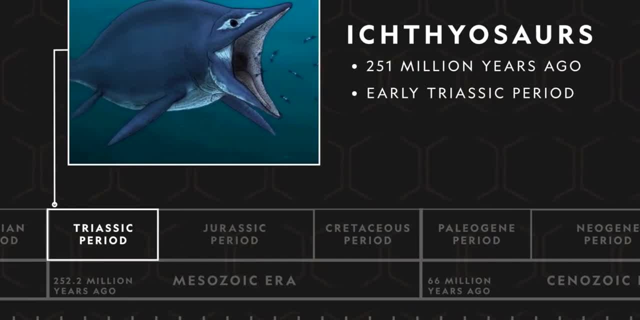 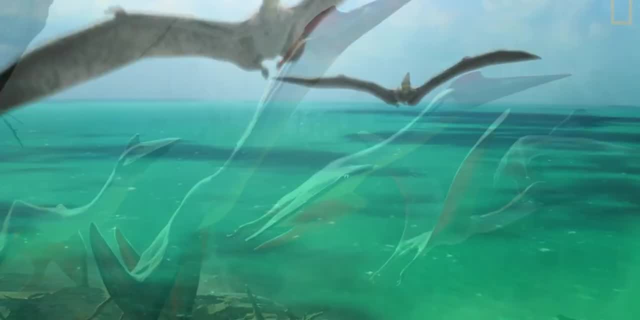 creatures such as the Ichthyosaurs, marine reptiles resembling dolphins, and the long-necked fish-eating Tanistropheus. The skies, on the other hand, saw the presence of Pterosaurs, the first flying vertebrates, These early Pterosaurs. 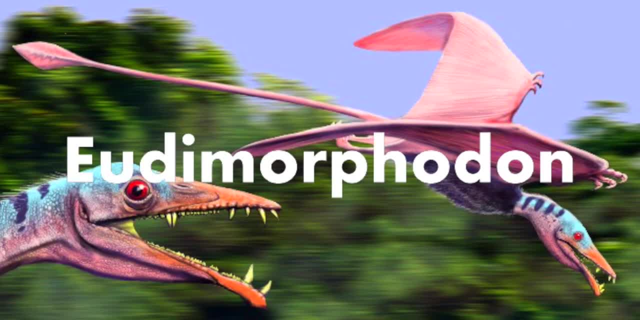 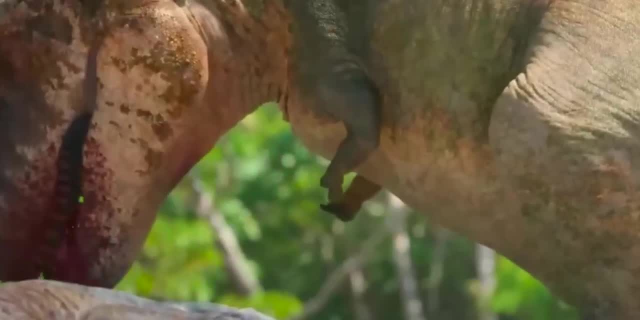 like the Eudamorphodon, possessed the ability to soar through the air and played a crucial role in the early history of flight. These fascinating creatures set the stage for the extraordinary diversity of life that would come to define the later periods of the Mesozoic era. The landmasses during the Triassic period were different from what we see today. The supercontinent Pangea continued to exist, although it started to break apart during this period. This fragmentation led to the formation of new landmasses and oceans. 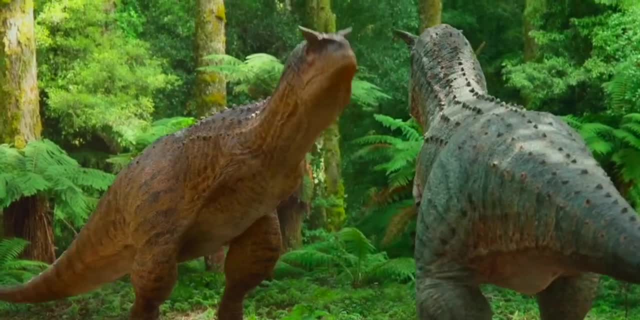 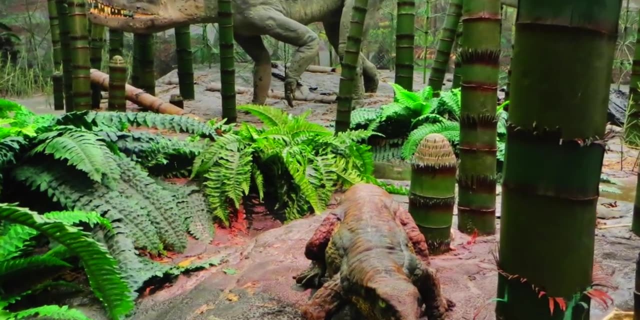 reshaping the planet's geography. The Triassic period also saw the proliferation of various plants, including ferns, conifers and cycads. These plants played a crucial role in establishing terrestrial ecosystems and providing habitats for the evolving animal life Throughout the 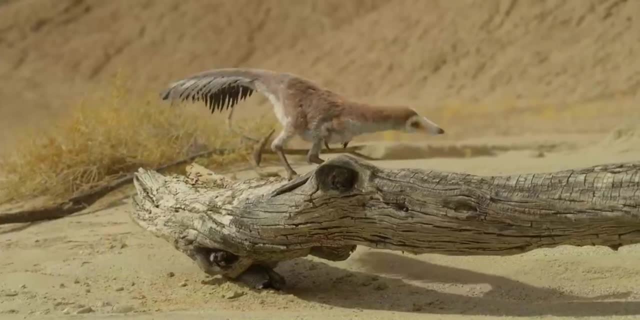 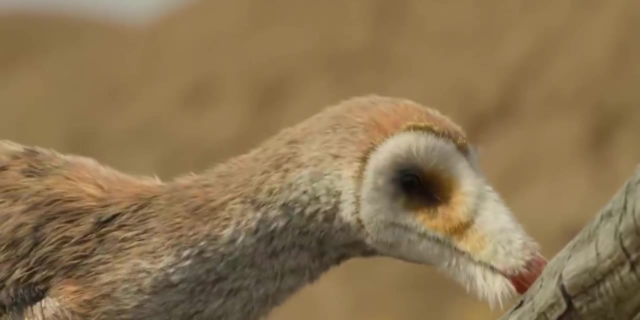 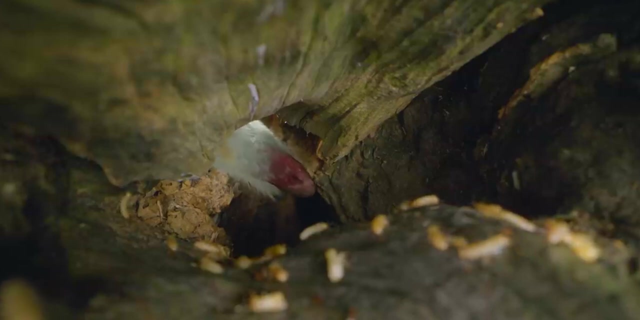 Triassic period, Earth experienced fluctuations in climate from relatively dry and arid conditions to more humid and tropical environments. These changing climatic conditions influenced the distribution and evolution of organisms during this time. While the Triassic period was a time of recovery and innovation, it eventually set the stage for 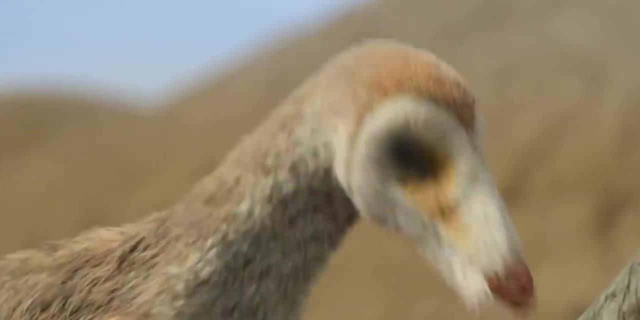 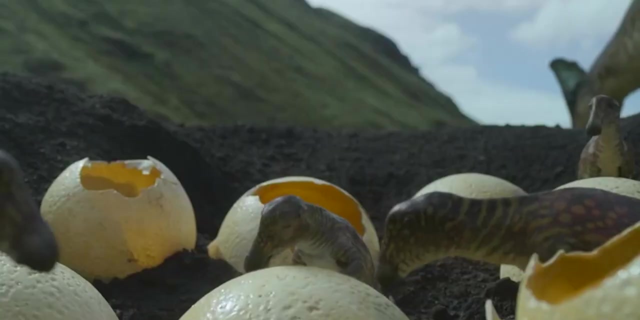 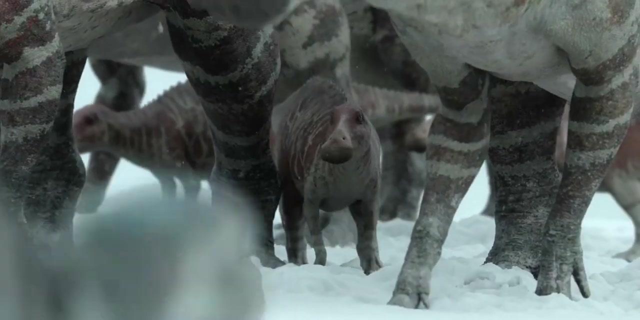 the subsequent periods of the Mesozoic era. The diverse reptilian lineages that emerged during this period would continue to evolve and dominate the planet during the later Jurassic and Cretaceous periods. The Jurassic period- The Jurassic period spanning approximately 201 million years ago to 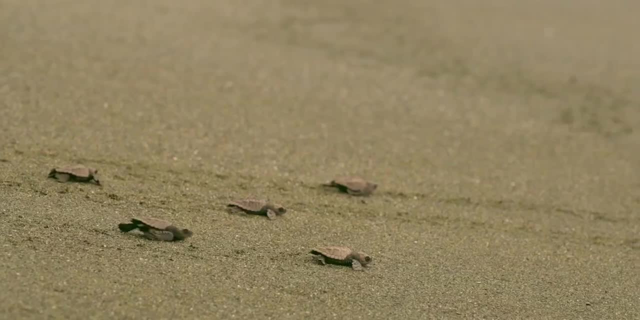 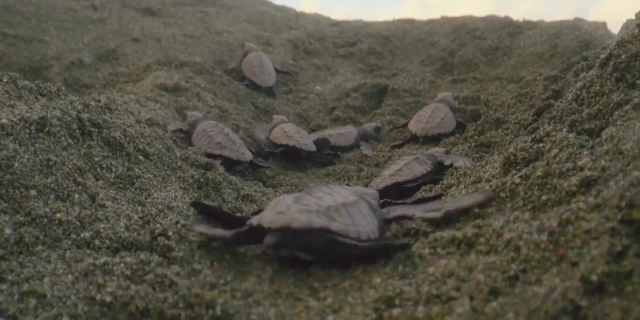 145 million years ago stands as one of the most iconic and captivating chapters in Earth's history. It was a time of immense biodiversity and the zenith of the age of dinosaurs. The landmasses continued to shift, with the supercontinent Pangea slowly breaking. 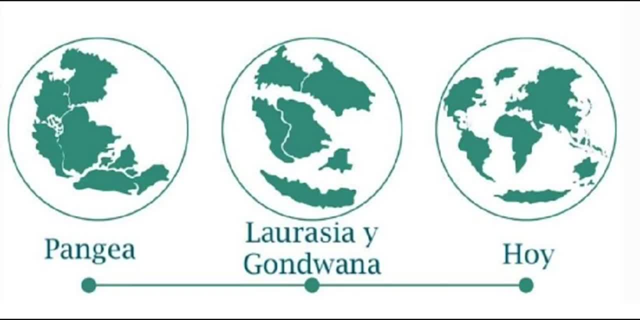 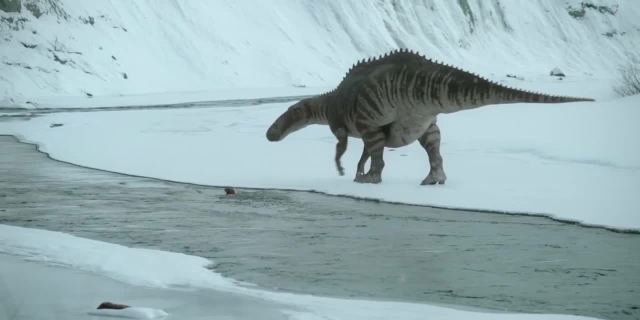 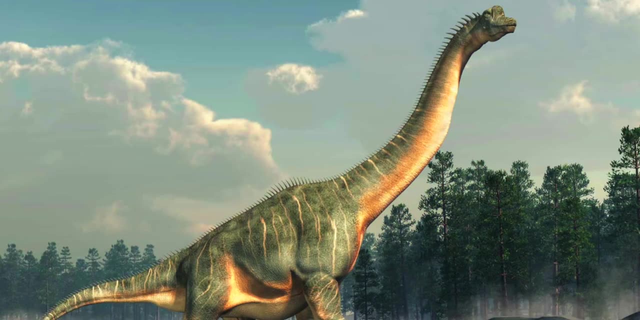 apart, leading to the formation of new continents and oceans. As the continents separated, diverse environments emerged, from lush forests to vast desert regions. During the Jurassic period, dinosaurs reigned supreme, showcasing an astonishing array of sizes, shapes and behaviors. Majestic. 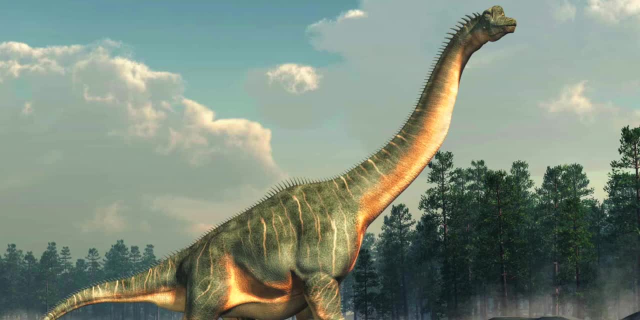 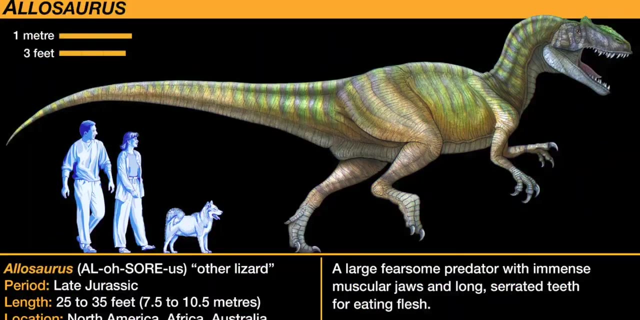 herbivorous dinosaurs were able to survive in the vast deserts of the Earth, and their long-necked brachiosaurus and diplodocus roamed the ancient landscapes, utilizing their enormous size to graze on abundant vegetation. Meanwhile, formidable predators such as the Allosaurus and 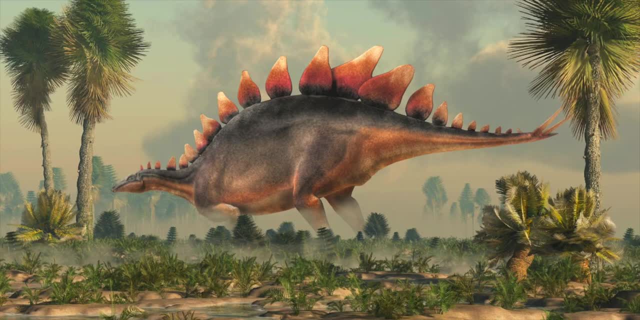 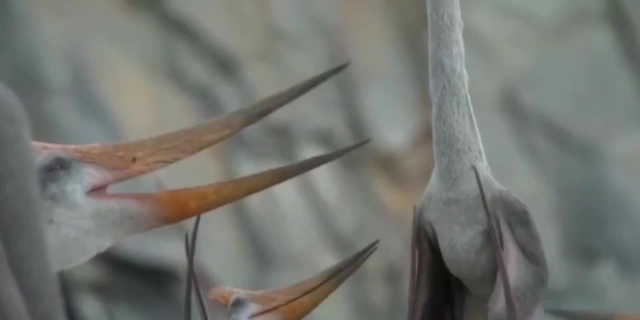 the iconic Stegosaurus roamed the land, employing various hunting strategies to secure their prey. It was during this period that the first birds evolved from small theropod dinosaurs, marking a pivotal moment in the history of life on Earth. These early avian creatures 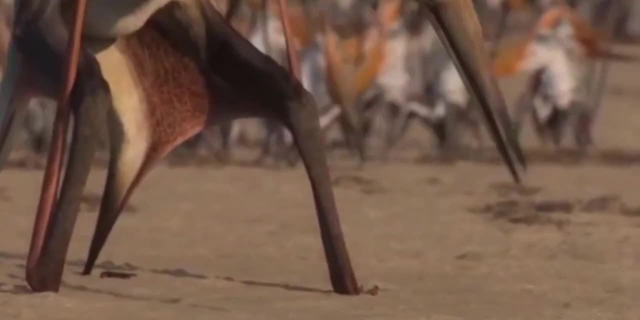 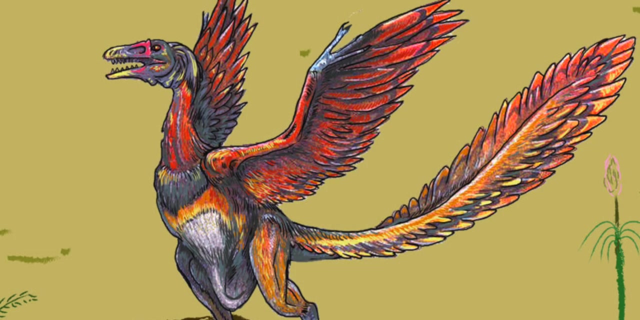 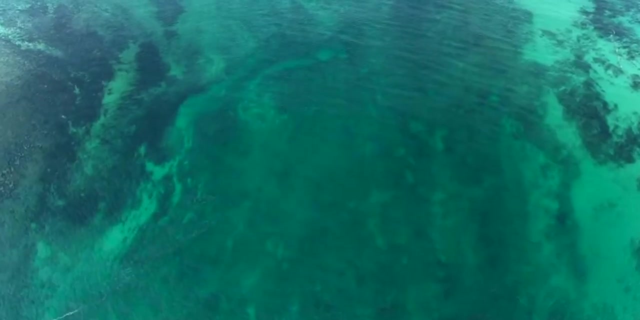 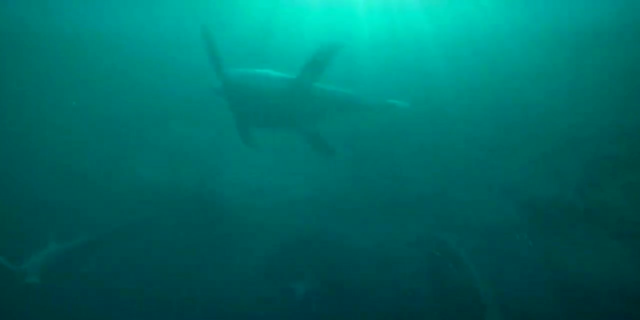 like Archaeopteryx, possessed both reptilian and reptilian abilities. The first bird to be born was the Archaeopteryx, a species of reptilian and avian characteristics showcasing a transitional form between dinosaurs and birds. The presence of these ancient birds offers a fascinating 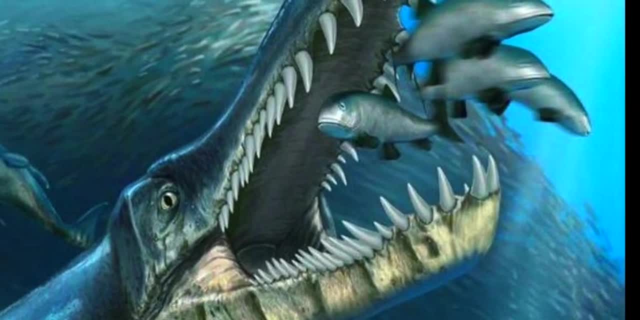 glimpse into the evolutionary link between reptiles and modern avian species. The seas of the Jurassic period were teeming with life. Marine reptiles like the long-necked plesiosaurs and the swift ichthyosaurs dominated the oceans, while the fearsome marine predators, such as the powerful marine crocodiles known as metriorhynchids, patrolled the waters. 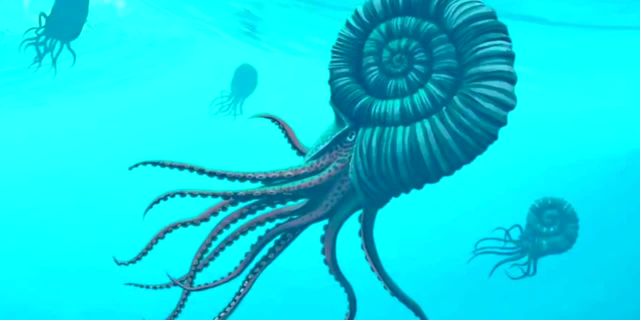 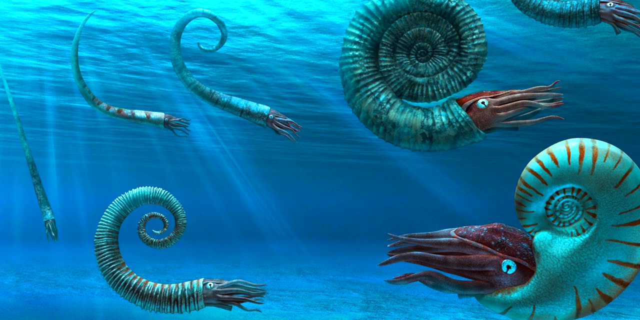 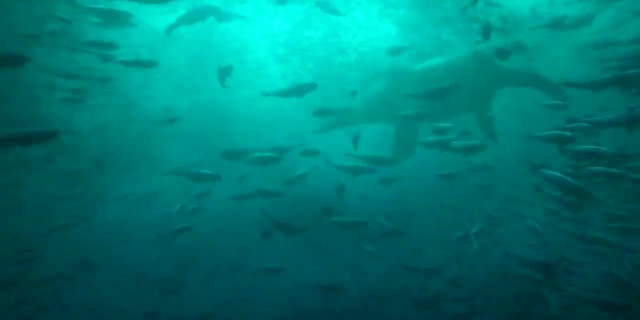 In addition to reptiles, various species of ammonites, squid-like creatures with spiral shells, thrived in the oceans, leaving behind an extensive fossil record. The flora of the Jurassic period also underwent significant changes: Conifers, cycads and ferns continued to flourish. 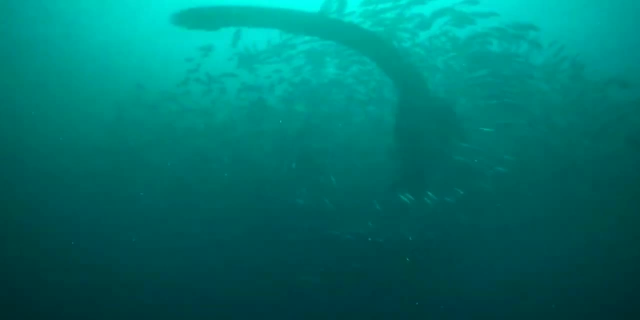 but the period saw the emergence and dominance of new plant groups, such as the widespread and diverse group of seed plants known as cicadioids. These plants played a crucial role in the shaping the ecosystems of the time and providing habitats for a wide range of organisms. 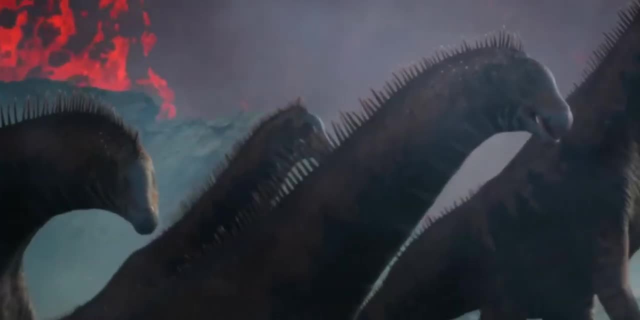 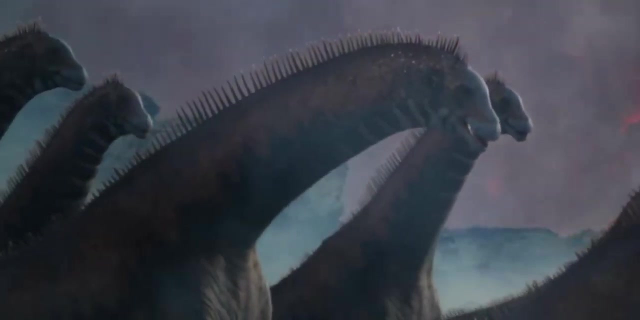 The Jurassic period came to an end with several notable events, including volcanic activity, climatic fluctuations and shifts in sea levels. These factors set the stage for the next period of the Mesozoic era, the Cretaceous period, which would witness even greater changes and bring 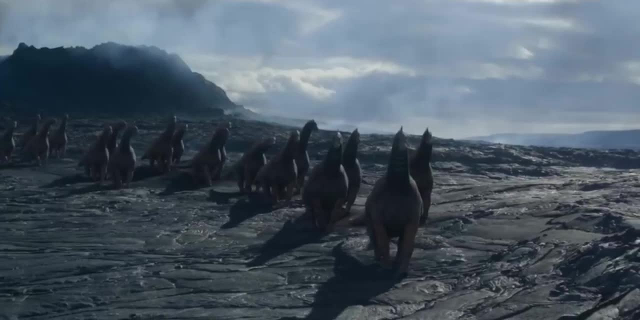 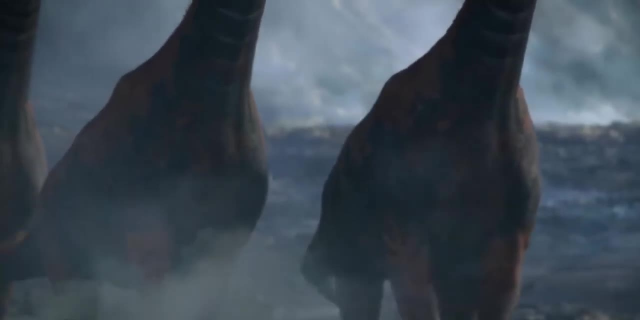 forth new and extraordinary life forms. The Jurassic period holds a special place in our understanding of Earth's history. The caregiver, the habitat and the marine habitat are all captivating us, with its colossal dinosaurs, intriguing fossils and the evolving story of life's continuous adaptation and diversification. 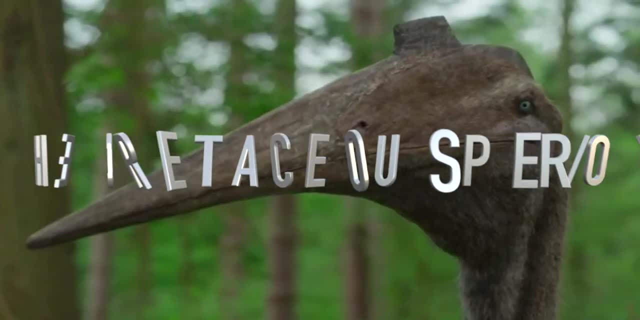 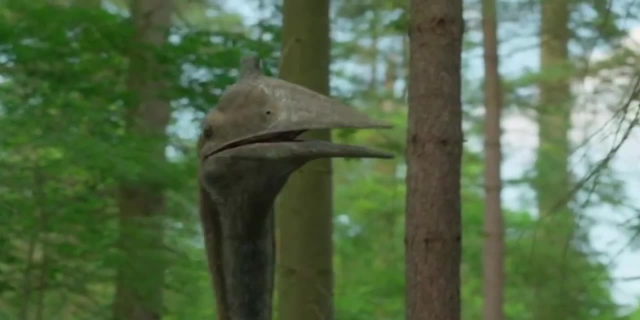 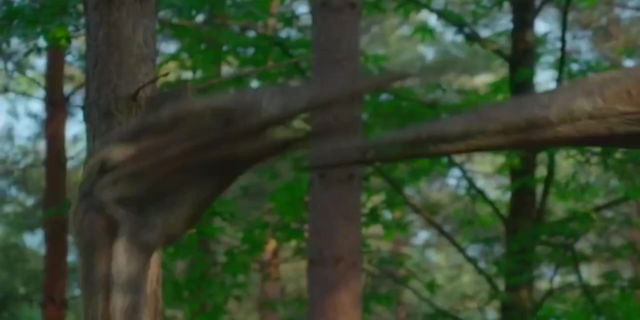 The Cretaceous Period. The Cretaceous Period, spanning approximately 145 million years ago to 66 million years ago, was a time of immense geological and biological transformations. It was the final period of the Mesozoic Era and witnessed the highest diversity and dominance of dinosaurs. The landmasses continued to shift, with the fragmentation of the supercontinent Pangea, resulting in the formation of separate continents and oceans. The Cretaceous Period was marked by the flourishing of diverse dinosaur species: Gigantic, herbivorous dinosaurs, such as the long-necked Argentinosaurus. 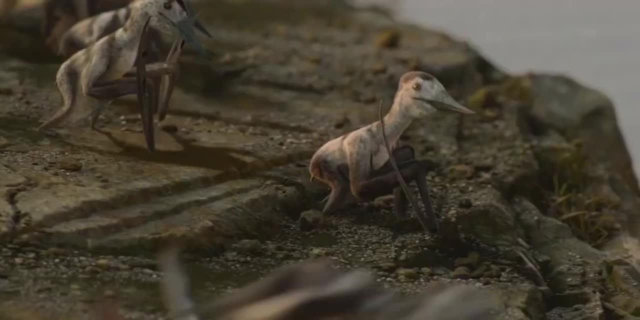 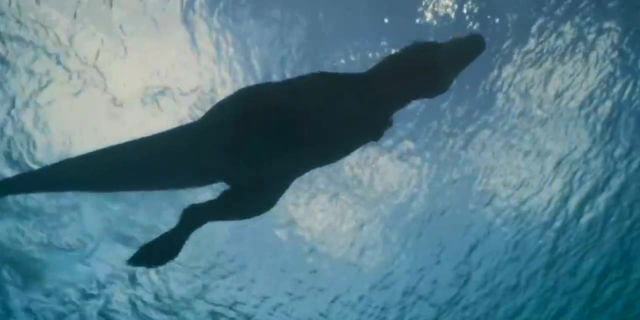 and the heavily armored Ankylosaurus roamed the ancient landscapes, adapting to the various environments. The theropod dinosaurs also continued to evolve, with the appearance of massive predators like the Iconoceros, the iconic Tyrannosaurus rex and the swift Velociraptor. 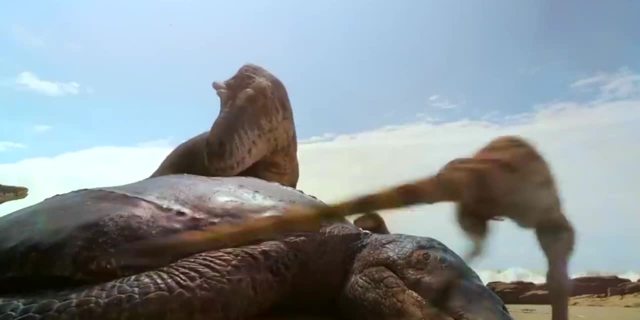 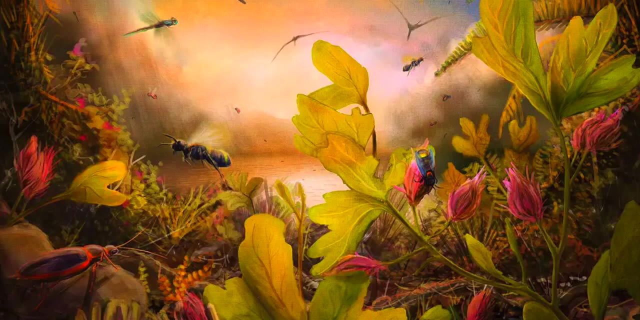 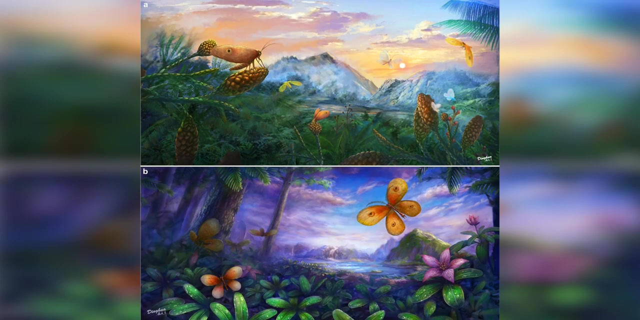 These fierce carnivores dominated the food chain, showcasing an exceptional display of adaptation and predatory prowess. Notably, the Cretaceous Period witnessed the evolution and diversification of flowering plants known as angiosperms. This botanical revolution resulted in the spread of diverse ecosystems. 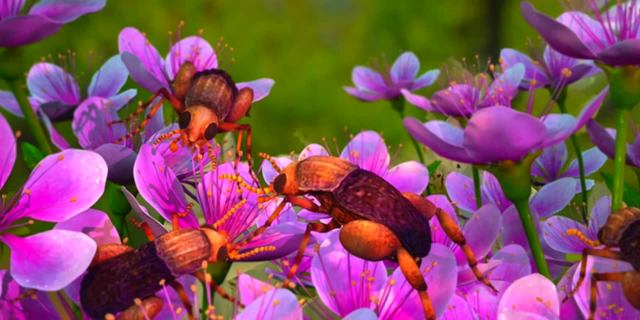 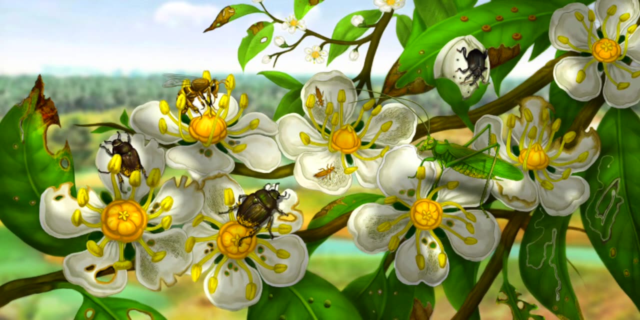 with colorful flowers and a wide array of fruits. The co-evolution of angiosperms and insects such as bees and butterflies played a crucial role in their successful propagation and pollination. The seas of the Cretaceous Period were home to an astonishing array of marine life. 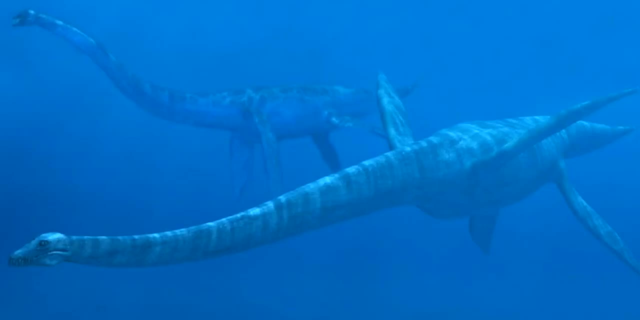 Marine reptiles, including the long-necked Elasmosaurs and the large predatory Mosasaurs, ruled the oceans with their unique adaptations. These reptilian behemoths navigated the prehistoric waters, capturing their prey with specialized jaws and teeth. 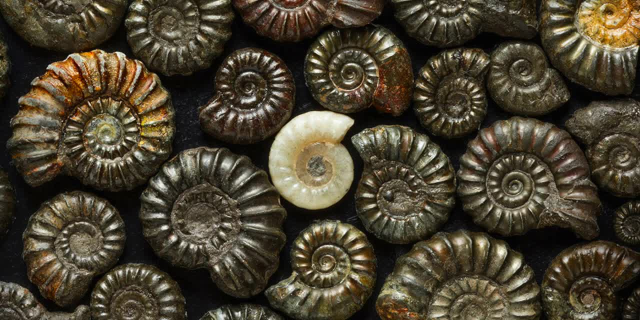 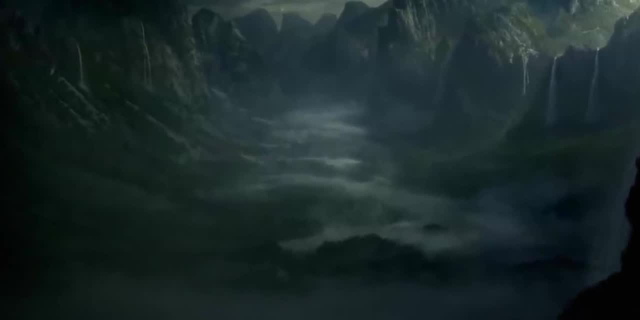 Additionally, the ammonites, a diverse group of marine cephalopods, continued to thrive, displaying intricate shell designs. However, towards the end of the Cretaceous period, a catastrophic event occurred, forever altering the course of life on Earth. 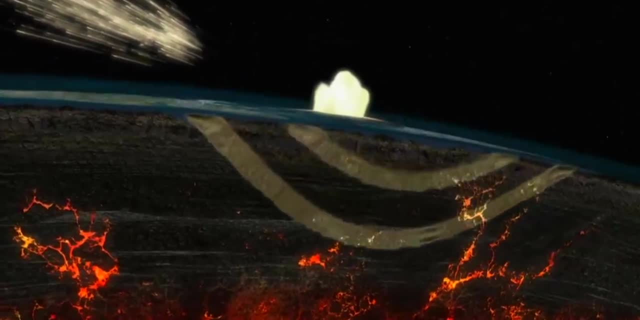 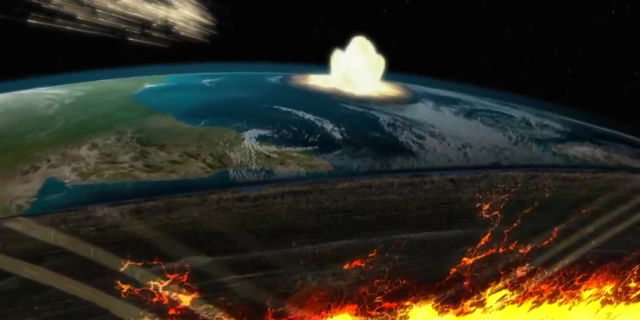 This event, known as the Cretaceous-Paleogene Mass Extinction Event, wiped out a significant portion of lifeforms on the planet, including the non-avian dinosaurs. The cause of this mass extinction event is widely attributed to a combination of factors. 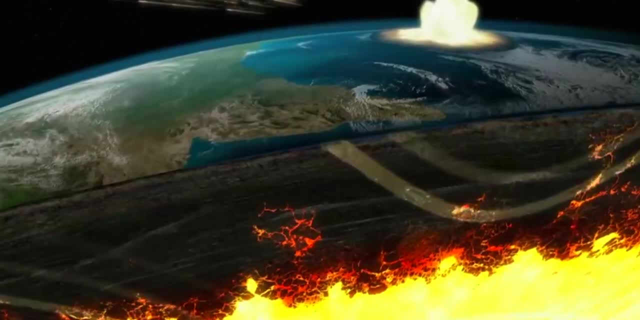 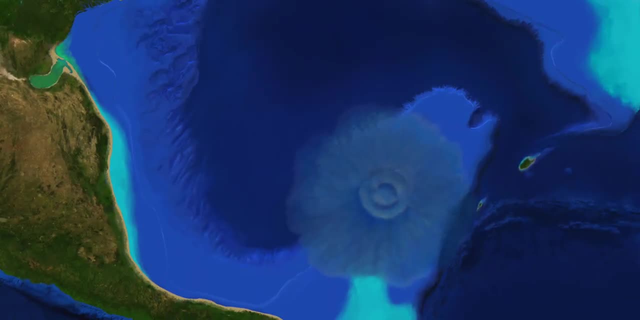 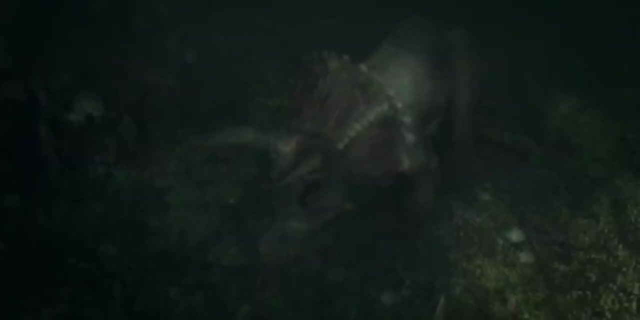 including intense volcanic activity, asteroid impact, climate change and environmental disruptions. The impact of an asteroid in what is now the Yucatan Peninsula in Mexico, known as the Chicxulub impact, is particularly believed to have played a significant role in triggering global-scale devastation. 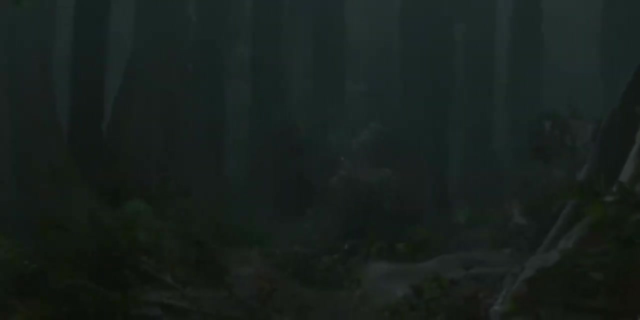 The resulting dust, debris and climate disturbances caused a dramatic decline in sunlight, leading to the collapse of ecosystems and the extinction of many species, including the mighty dinosaurs. The Mass Extinction Event at the end of the Cretaceous period marked a turning point in Earth's history.